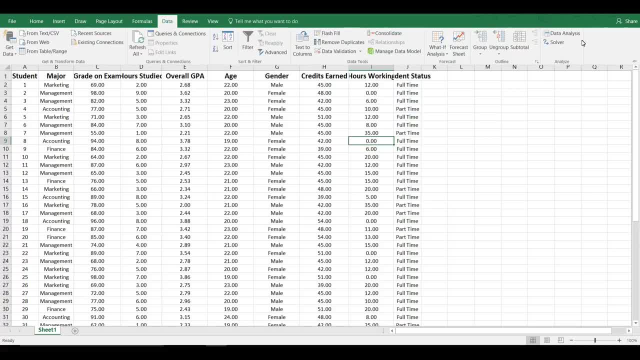 that's it Now. when you look under the data tab, you will see on the ribbon the data analysis tool. If it isn't there at this point, I would shut down Excel and restart it. You just have to do this one time. Once it's installed, it is there. So now let's use the data analysis. 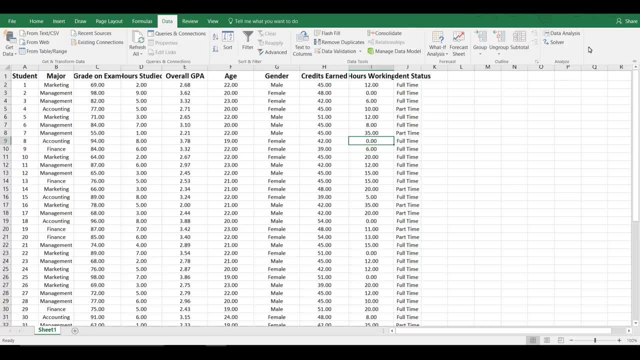 tool to run descriptive statistics on one of the variables in this worksheet. I have student major grade on exam. Alright, let's do grade on exam. Grade on exam is the C column, And so, in order to run descriptive statistics on this C column, we go to the data analysis. 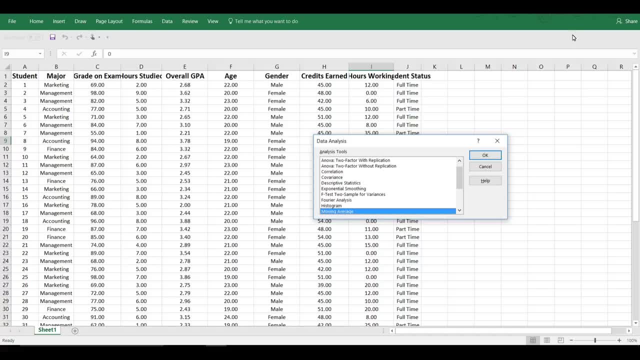 tool. Once the dialogue box comes up, you can see all the analysis tools that there are. I can scroll down and you can see all the possible choices here, But what we want to do is something very simple, and that is descriptive statistics. So click on descriptive. 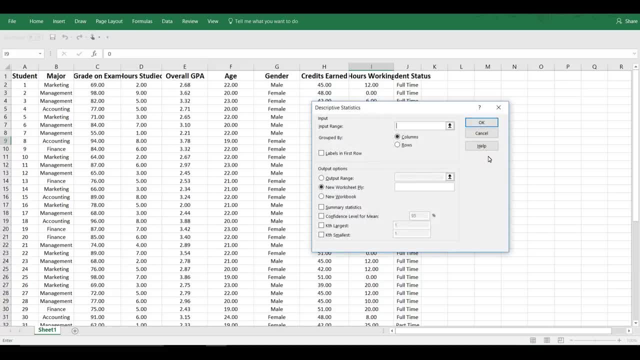 statistics. then click okay and now you have the descriptive statistics dialogue box. We have the input range. alright, We want the C column and there are two ways to do that. could type in c1 through 51. okay, you can see, the last row is 51, so we could type: 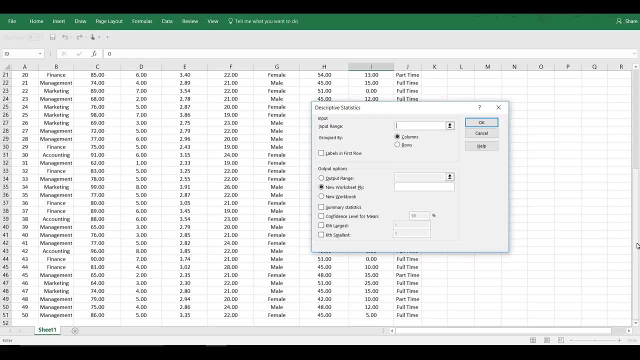 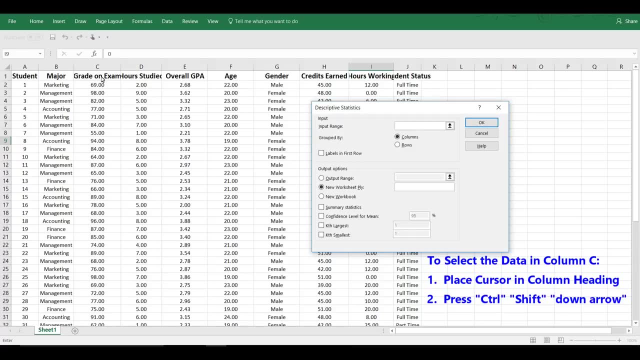 in c1 through 51. we could scroll and highlight it, or we can do a simple shortcut that works very well and that is, put the cursor in this heading. there we go the cursors in the heading and now press the ctrl, shift and down, key down. 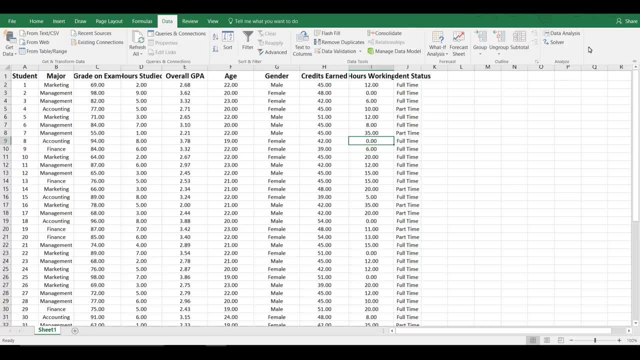 tool to run descriptive statistics on one of the variables in this worksheet. I have student major grade on exam. Alright, let's do grade on exam. Grade on exam is the C column, And so, in order to run descriptive statistics on this C column, we go to the data analysis. 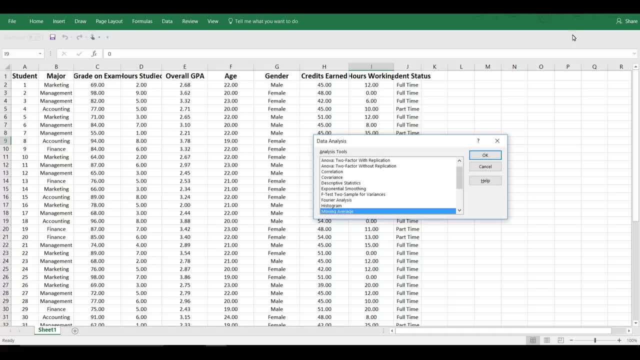 tool. Once the dialog box comes up, you can see all the analysis tools that there are. I can scroll down. you can see all the possible choices here, But what we want to do is something very simple, and that is descriptive statistics. So click on descriptive statistics, then click. 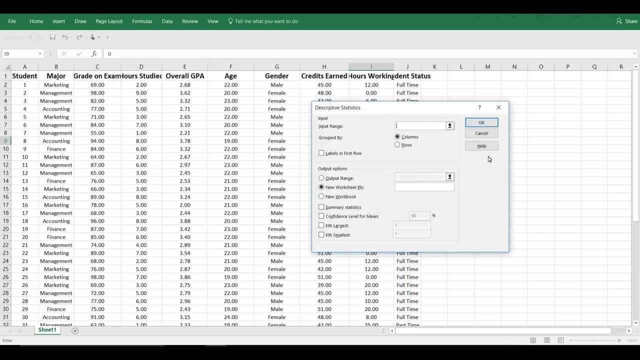 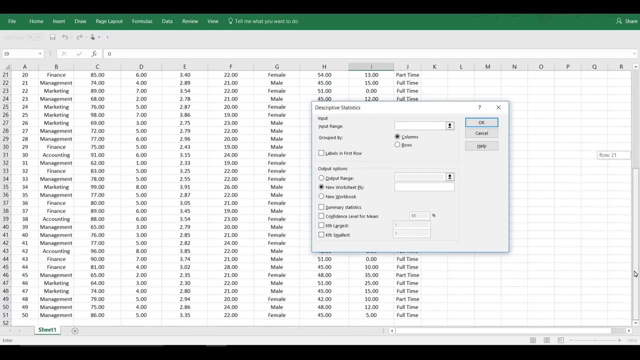 ok, And now you have the descriptive statistics dialog box. We have the input range. alright, We want the C column, And there are two ways to do that. We want the C column and there we could type in c1 through 51. okay, you can see, the last row is 51, so we could type in c1 through. 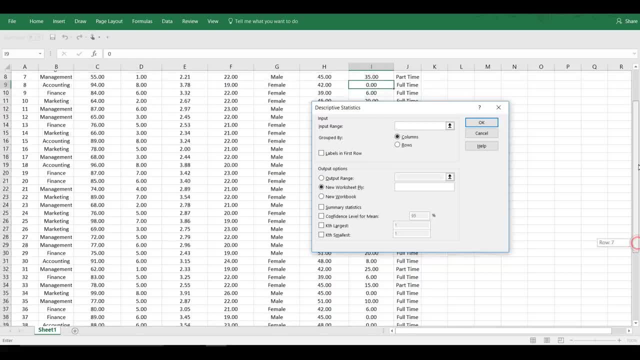 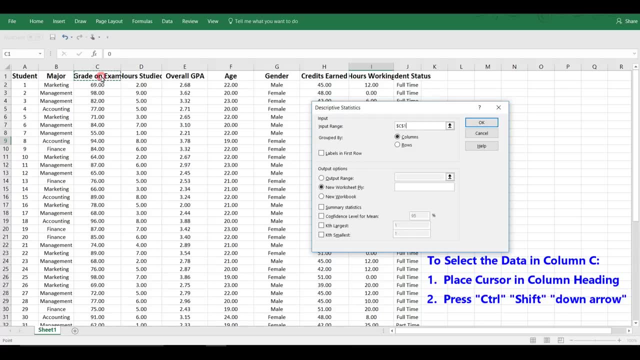 51. we could scroll and highlight it, or we can do a simple shortcut that works very well and that is put the cursor in this heading. there we go, the cursor is in the heading and now press the control, shift and down, key down at the same time, and it will automatically highlight all the data in that. 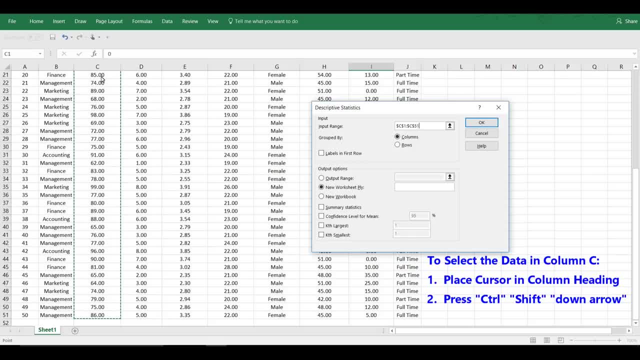 at the same time, and it will automatically highlight all the data in that row, and so you can see now it is c1 through c 51 as the input range. now let's check off labels in the first row, and the reason I did that is that we do. 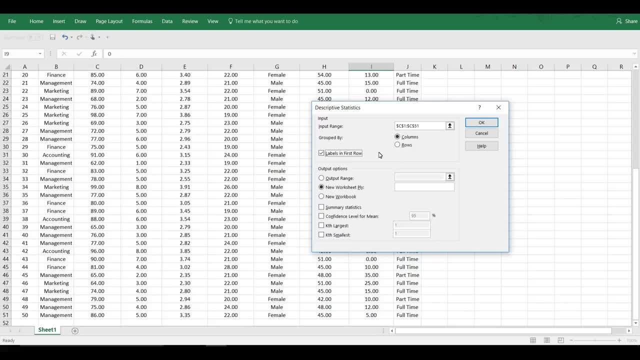 have labels. in the first row we have grade and exam as a label, and then for output range. I'm going to use a new worksheet: click on or check off summary statistics, because that's what we want. and then over here we have the kth largest and the 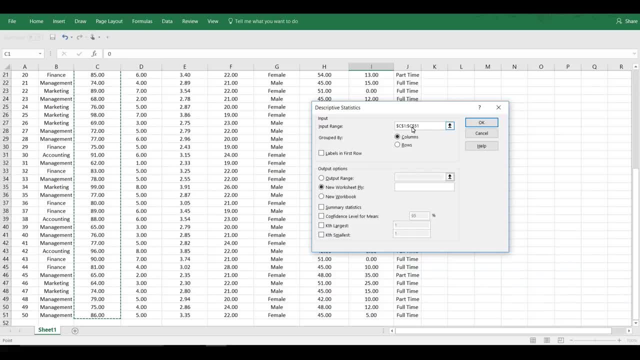 row, and so you can see now it is c1 through c51 as the input range. now let's check off labels in the first row, and the reason I did that is that we do have labels in the first row. we have grade, an exam as a label, and then for output range I'm going to use a new worksheet and then I'm going to 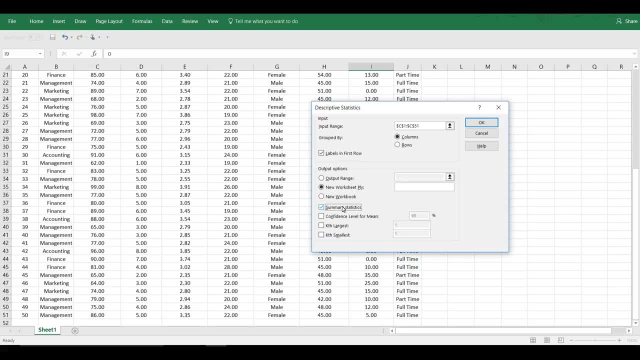 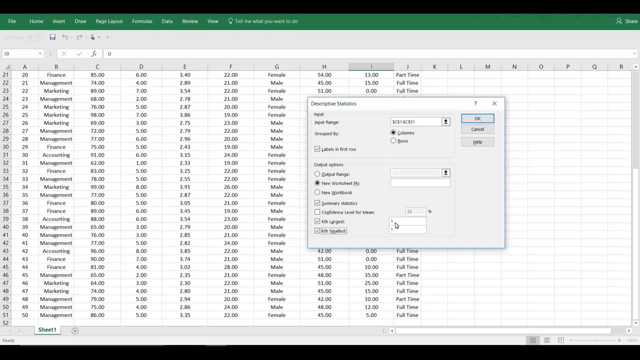 click on or check off summary statistics, because that's what we want. and then over here we have the kth largest and the kth smallest. so let's click kth largest and kth smallest now, by default it's the first largest. well, the first largest is the largest number in a data set, so that's the max, or? 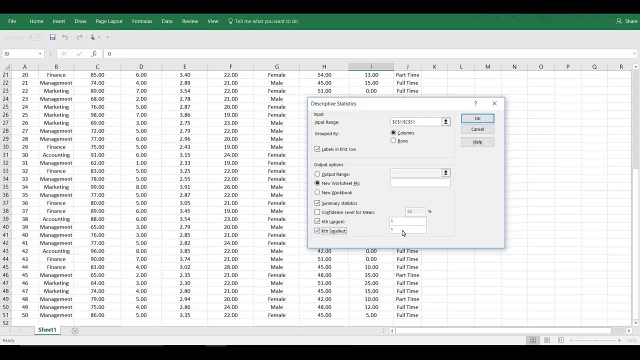 maximum and the kth smallest, by default is one that would be the one or first smallest, and so that's, of course, the minimum. well, descriptive statistics are the same as descriptive statistics already give you the maximum and the minimum, so I'm going to change that to a two. let's put a two.